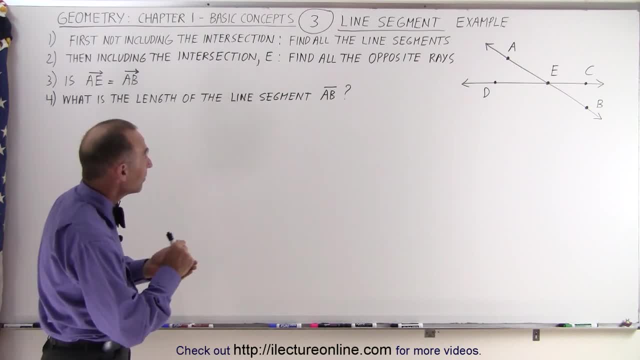 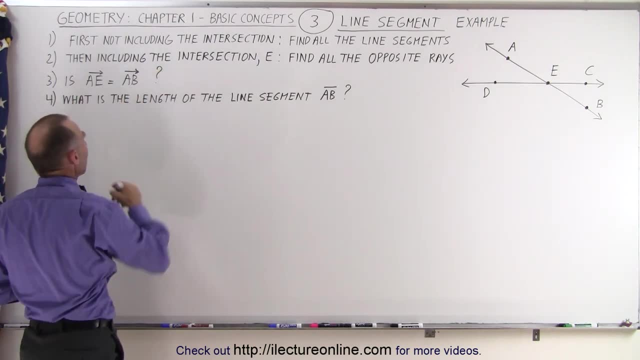 intersection, so including E, find all the opposite rays. Then we're going to ask the question and answer the question: is AE equal to AB? And so we have to understand what these symbols mean. And finally, what is the length of the line segment AB? And notice, here we have AB to an arrow. 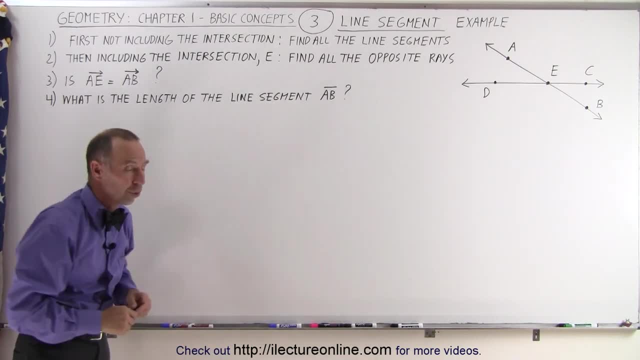 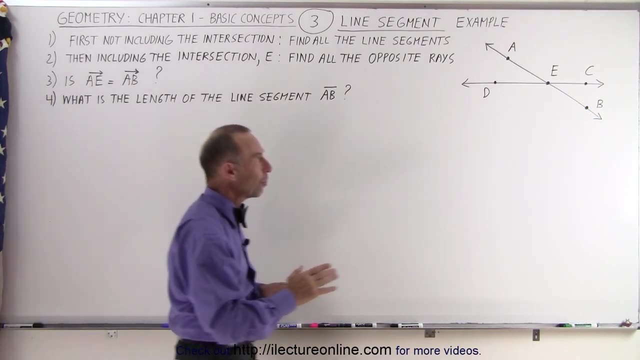 there we have AB with just a line on top, no arrow involved. So what do those symbols mean? What do we do with them? How do we answer those questions? So first, we're going to act as if the point E doesn't exist. We realize that this is the intersection of these two lines. 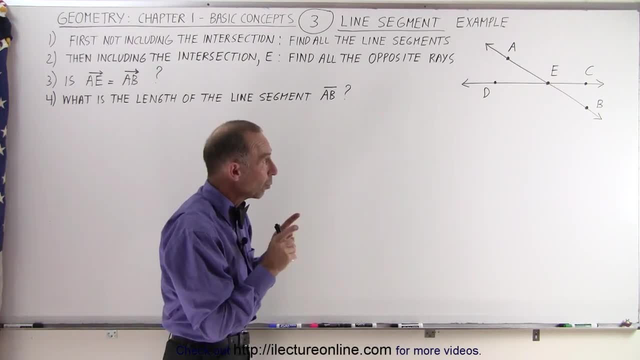 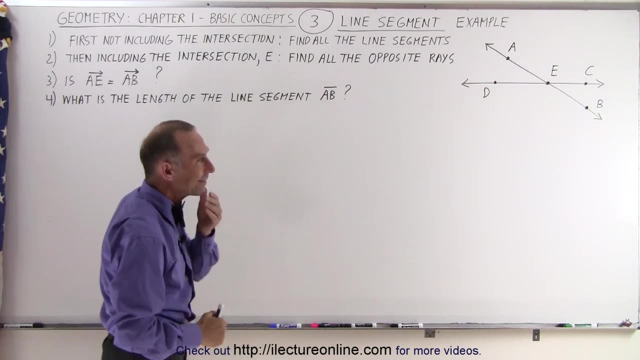 notice. we know their lines because they have arrows drawn on the ends, which means they go out to infinity. So we're supposed to find, ignoring E, all the line segments. Now, line segments are pieces of a line that are delineated, that have endpoints, and those endpoints are: 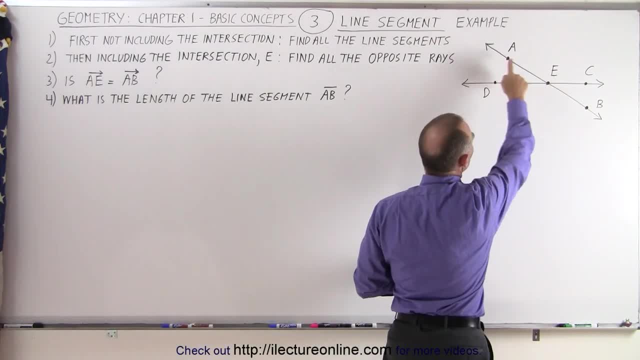 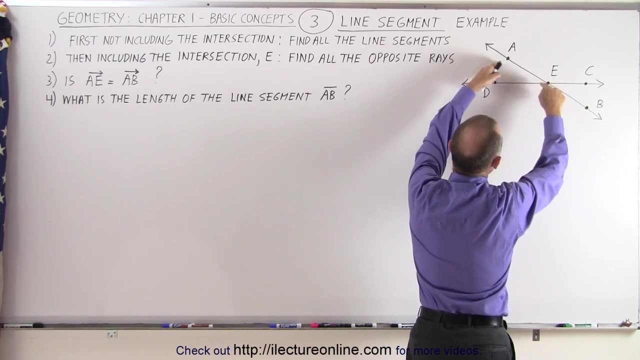 labeled by points. So here we have a point A, there we have a point B. So the line segment, the section of the line of this line right here that runs through the points A, E and B, this section here can be considered a line segment. And how do we denote that? We denote: 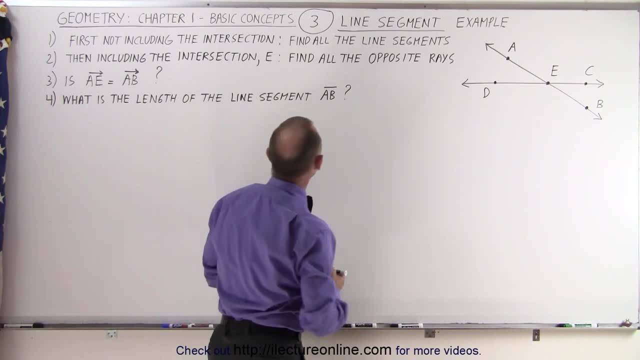 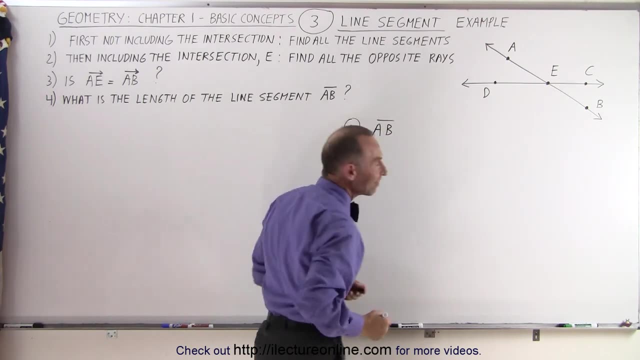 that with simply the two letters and a line on top. So for answer number one, we can say that A to B is a line segment, and so we put a line on top of that- We're ignoring the point E- And then we can see the other line. we have two endpoints. we have an endpoint here. 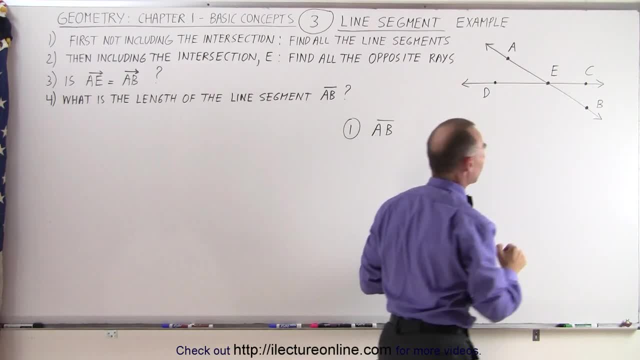 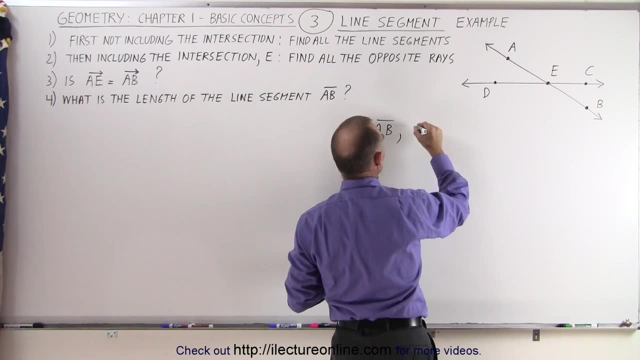 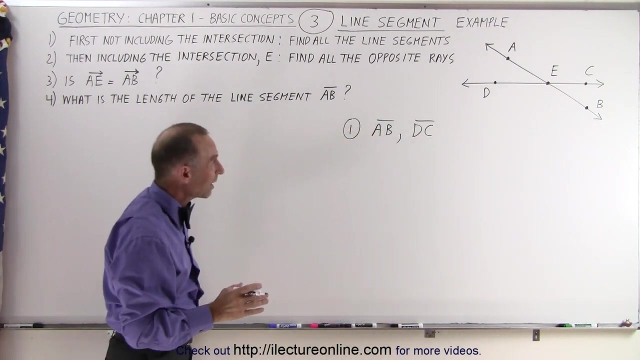 an endpoint there of that piece of the line, that section of the line that's called a line segment And therefore we can say, yes, that is also a line segment. So A, B and D, C would also be a line segment. Now could we write B, A and C- D? Yes, we could. We can say that A, B 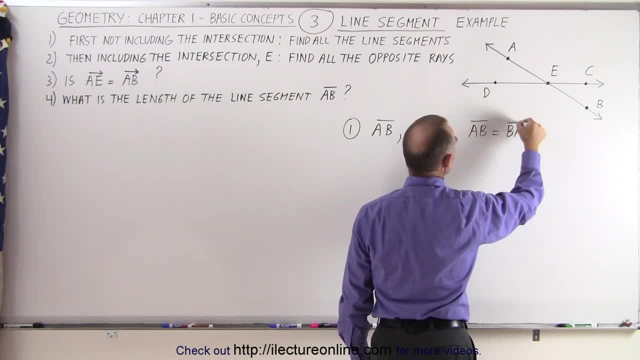 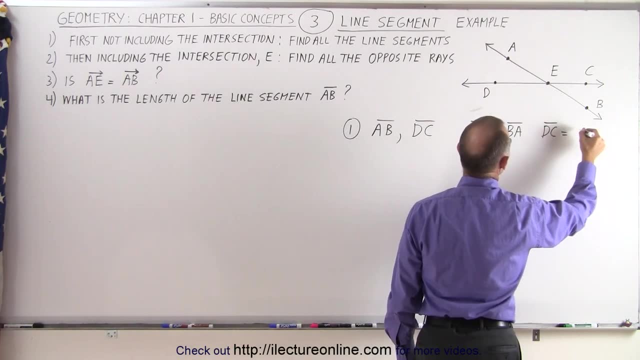 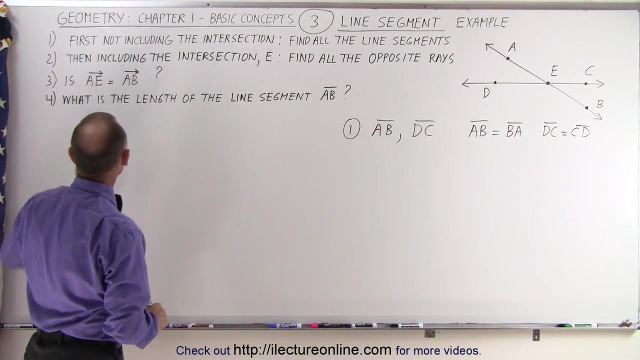 the line segment is the same as B A. It doesn't matter which letter you put first, it means the exact same thing. And we can write that D C is equal to C D. So it just means exactly the same thing. All right for number two. 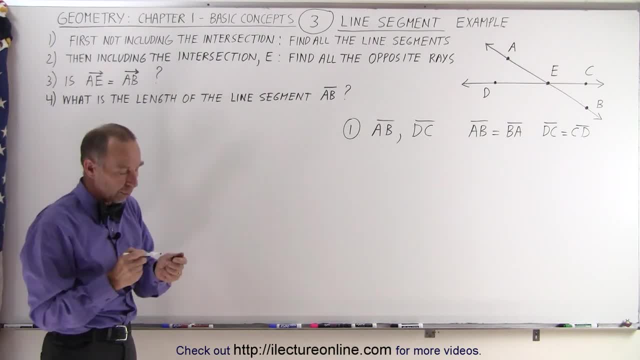 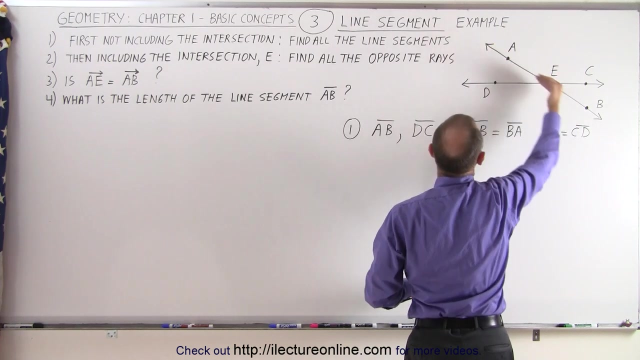 now including the intersection, find all the opposite rays. Remember, a ray is a piece of a line that has only one endpoint and on the other side it goes on to infinity. So we can say that, starting from E, we go to the point A and on to infinity. that would be a ray And starting. 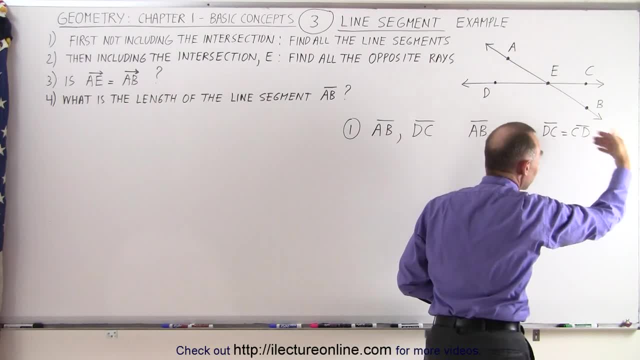 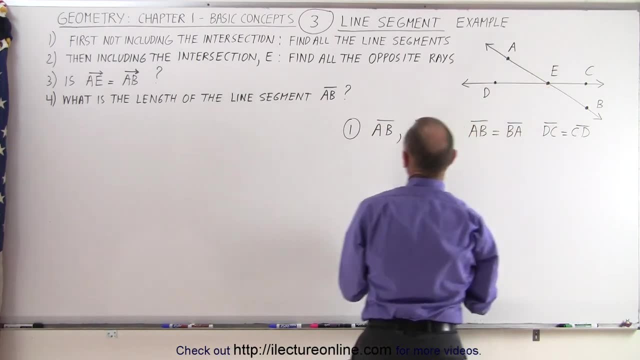 from the point E, going through B, going to the other side, that would be a ray, And so we can opposite direction, that's another ray. since they go in opposite directions and they start from the same point, then those would be two opposite rays. so the first opposite ray, the first one, could be: 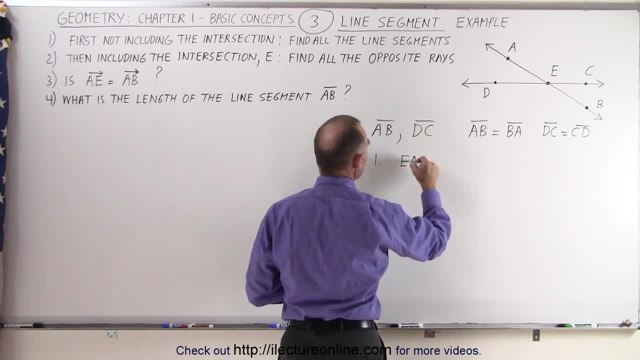 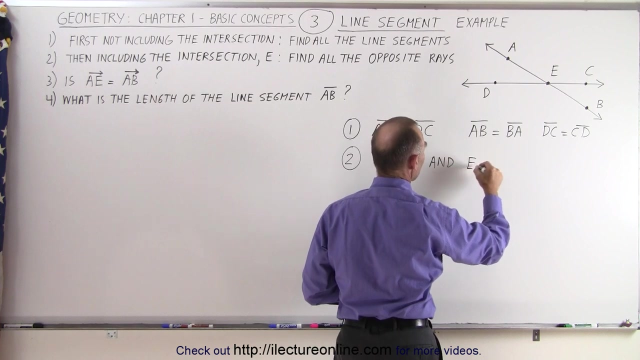 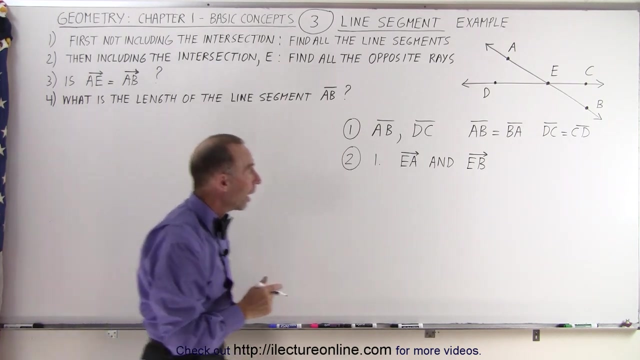 explained as e- a with an arrow on top, like that. that means this is a ray because it only has an arrow on one side, not on the other side. the end point is at e and we could start from e and go to b and on to infinity. so we draw a little arrow on top of it. so those two, e a and e b, are opposite rays. 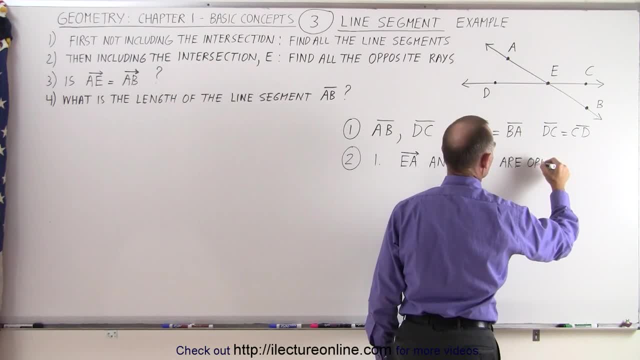 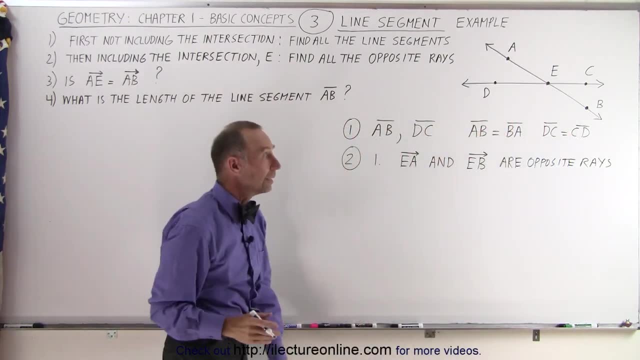 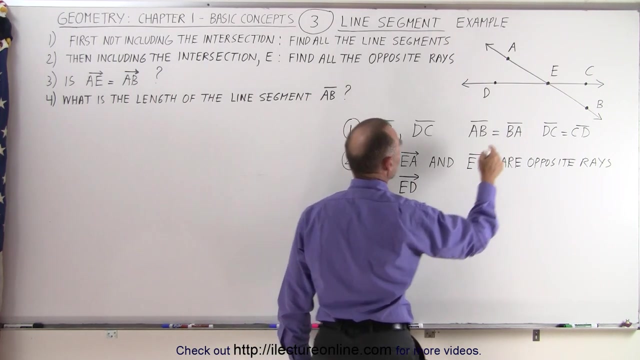 then if we look at the other line, we could do the same thing for the second pair. we can say: from e to d, that would be a ray, because that's the end point of one side. it goes through the point d and out to infinity. infinity in this direction. and if we don't again start at the point e and go in the opposite, 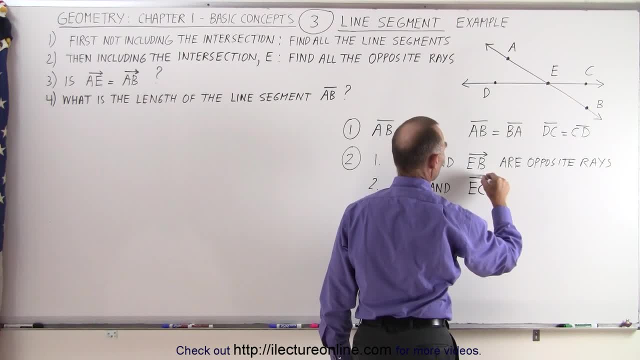 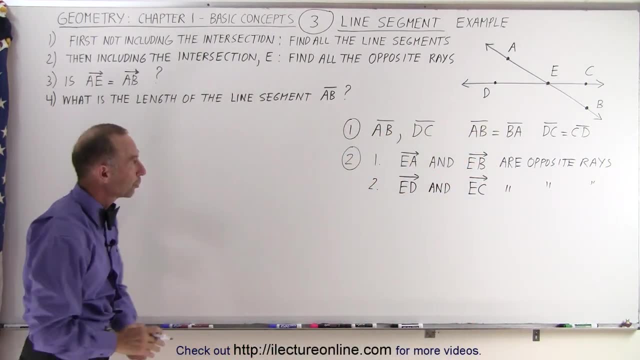 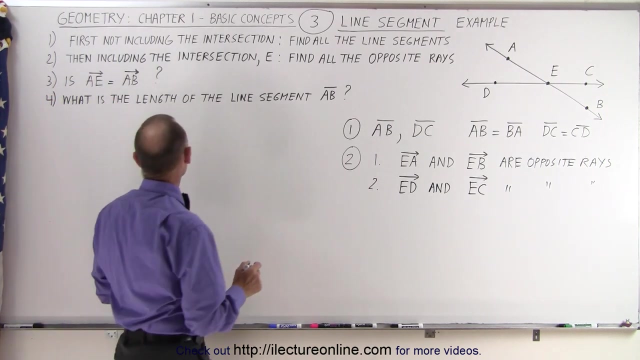 direction. through the point c, we're going to say ec with an arrow on top, and so we can say that are opposite rays as well. so that's the answer to number two. how about three? is ae equal to ab? that's interesting. let's take a look. first of all, we know that this is a ray because it has 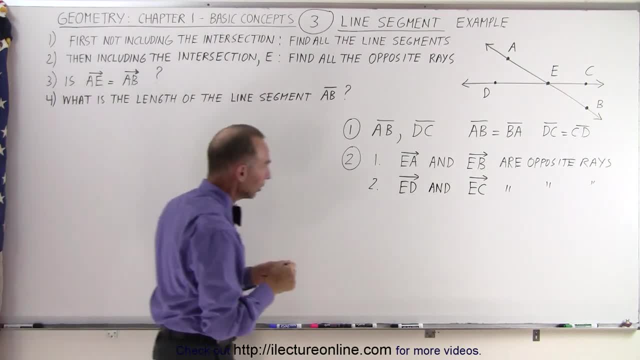 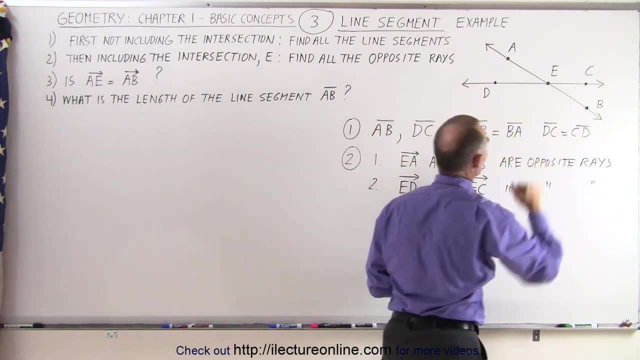 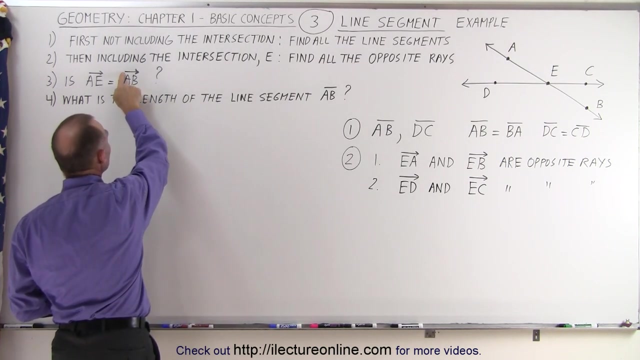 an arrow on one side and has an end point at a. so let's take a look, starting from a, that's the end point and it goes through the point e and then on to infinity. so that's a ray. what if we write it instead like this: ab notice, we have a starting point at a, or the end point that we 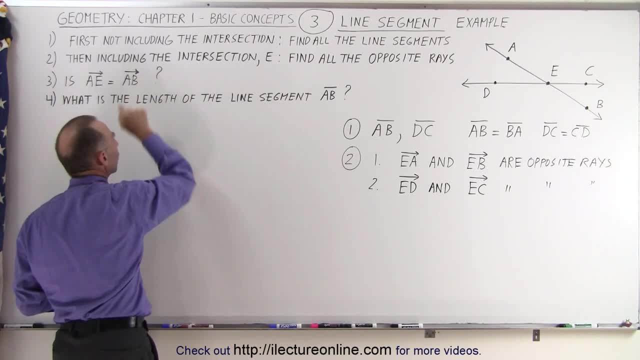 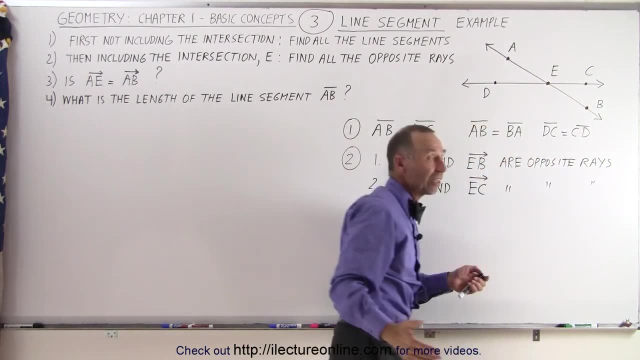 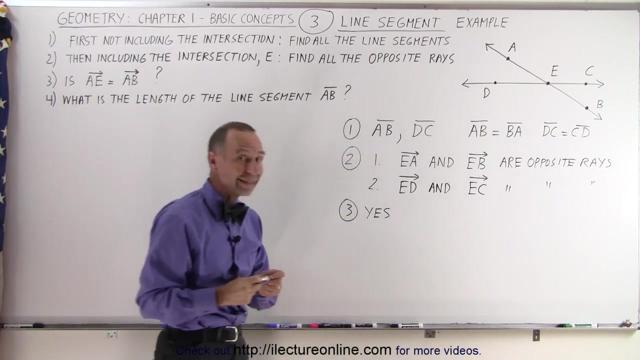 actually we should call an end point at a goes on to infinity. it goes to the point b- notice it has the same end point. it goes through e, through b and on beyond that. so essentially the answer, you, you is yes. for number three, yes, they are the exact same ray, just defined differently because there's